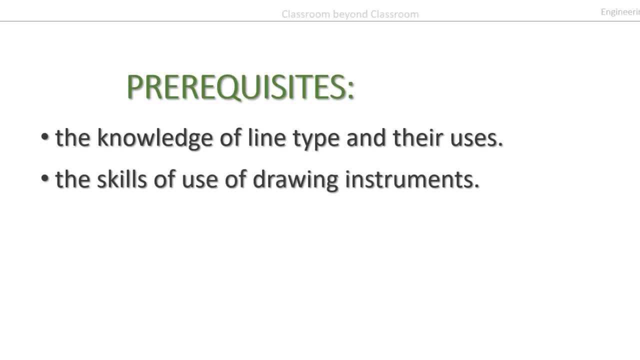 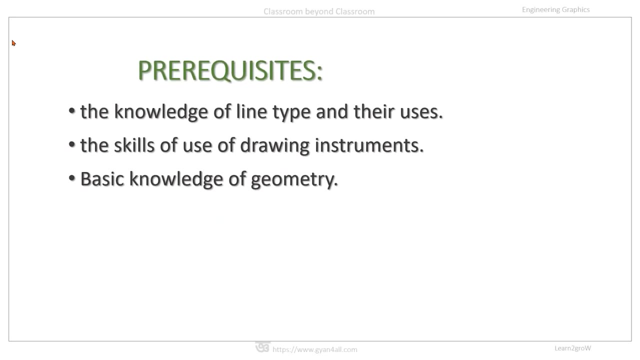 Learners should have the skills of using drawing instruments. For what purpose, which instrument is used, How to draw parallel lines, vertical lines, incline lines, and so on. Of course, geometrical construction requires the basic knowledge of geometry from the school levels. 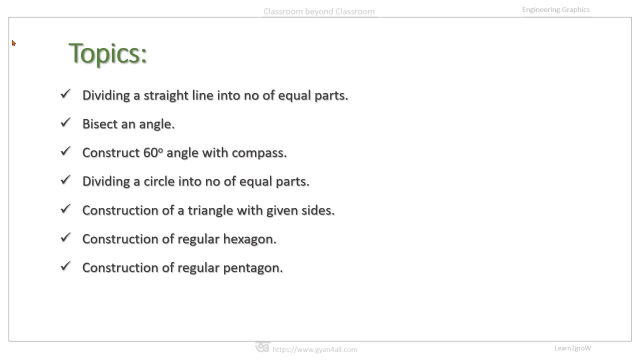 In this video we will demonstrate some of the basic construction methods, and this is not a complete list. but if these skills are developed, the learners can proceed for the next steps. The demonstration will be done using some virtual application software. The lines are drawn very 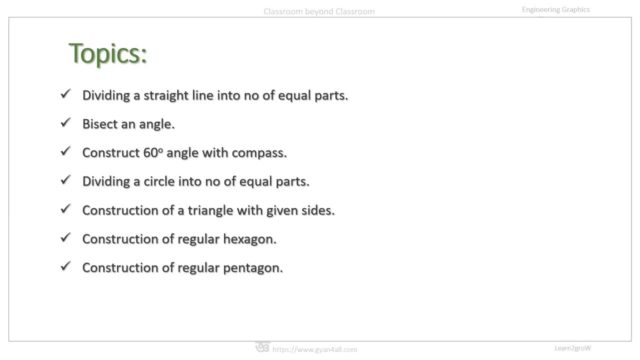 far away. The уА-А- tasks will be very difficult, But the Ua-Ж-Ғ- We will wait for the mission and then we are going to proceed. in this video, In today's video, we will nearly complete the application. 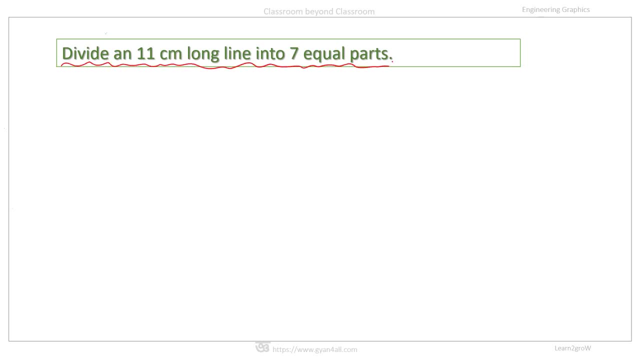 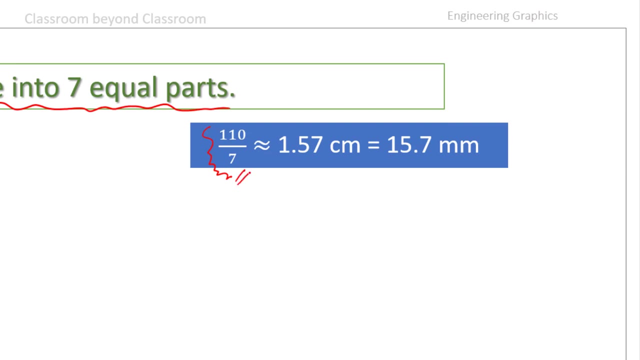 If necessary, if you are own sketch, you can pause the live video and then plan for your next design project or fill virtual application project. Next, Let's discuss about drawing of the lines of this shapes. We will start with the form. Let's start the drawing of the lines of the shapes which we have created, and that is 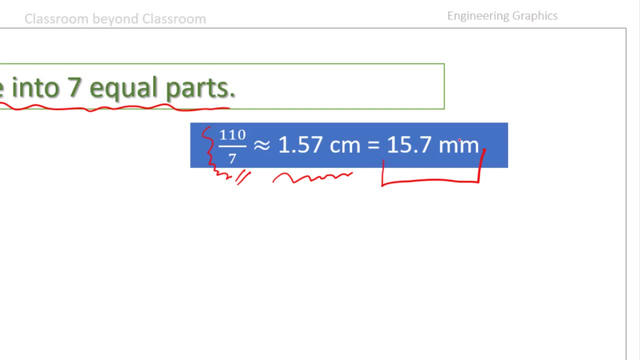 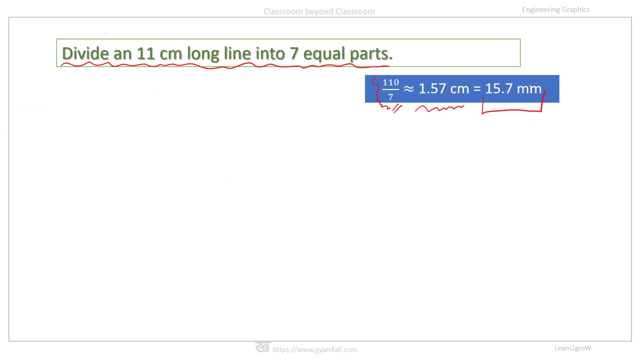 the section Q2-1 about drawing. Click on Follower & Mira for studies related to drawing. 画으뿡Lineae mark this distance. so we have to add up some other methods, which is extensively used in engineering drawing, and for that we learn the method of dividing a line. 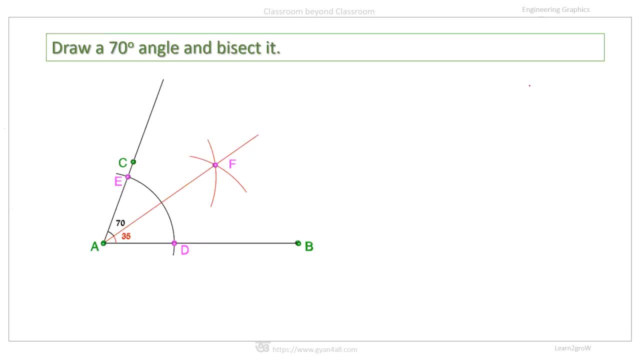 into equal number of parts. we will also draw a 70 degree angle and bisect it by using compass only. we will also construct a 60 degree angle with the help of compass and scales and we will divide a circle into equal number of parts and in our example, we'll divide the circle to 12- equal number of parts. 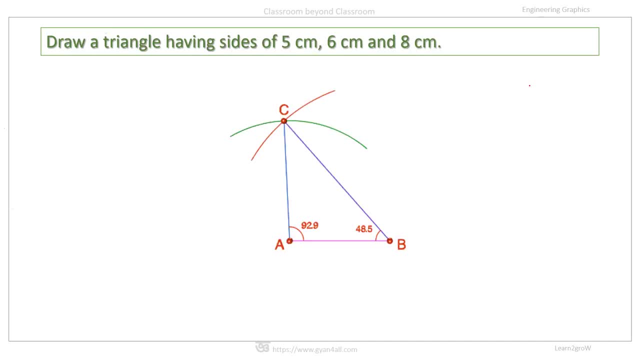 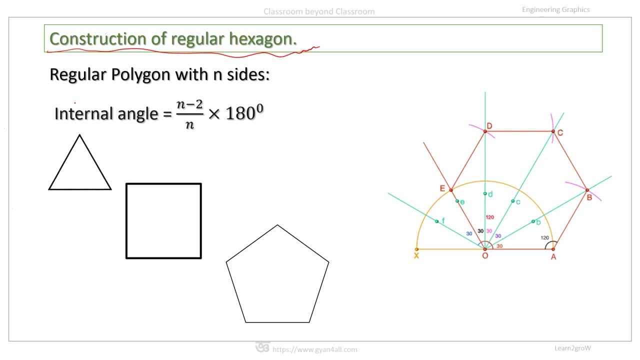 we'll draw a triangle with the help of compass and scale where the measurement of the sides are given 5 centimeters, 6 centimeter and 8 centimeter, and we'll also construct a regular hexagon with the given dimensions of the sides. say for a regular polygon, the n number of sides, the internal angle is. 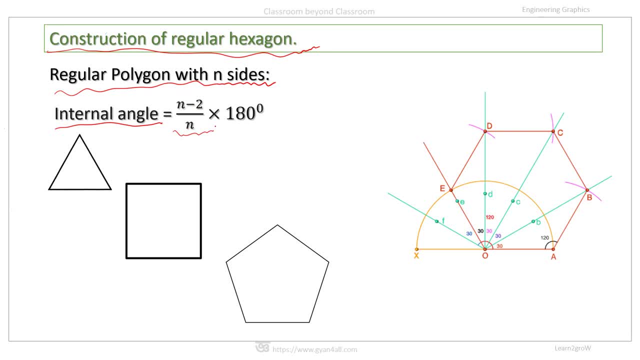 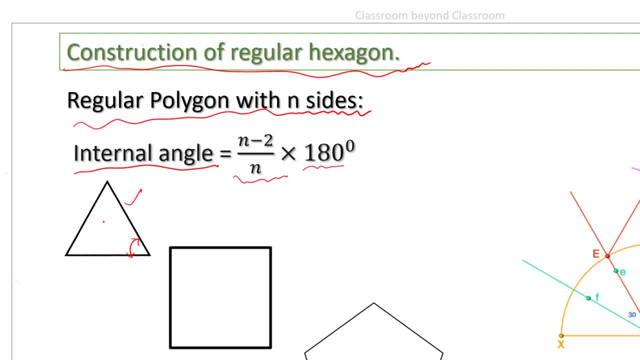 n minus 2 divided by n, multiplied by 180 degree. so for a triangle, if it is a regular polygon, then n is equal to 3, so the angle, internal angle, is 60 degree. for a square, which is a regular polygon, again n is equal to 4 and internal angle: 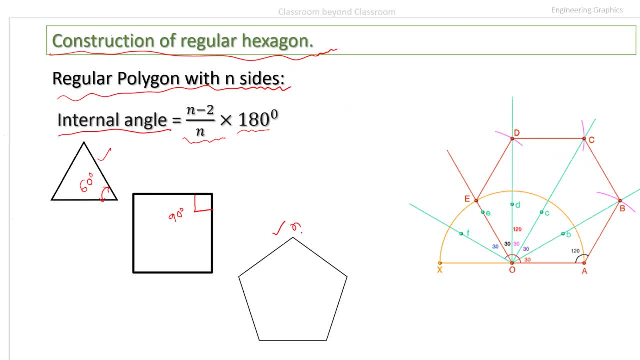 is equal to 90 degree for a pentagon. n is equal to 5, so the internal angle for a pentagon is equal to 100.. 108 degree. Similarly, for a hexagon, n is equal to 6, so it will give the internal. 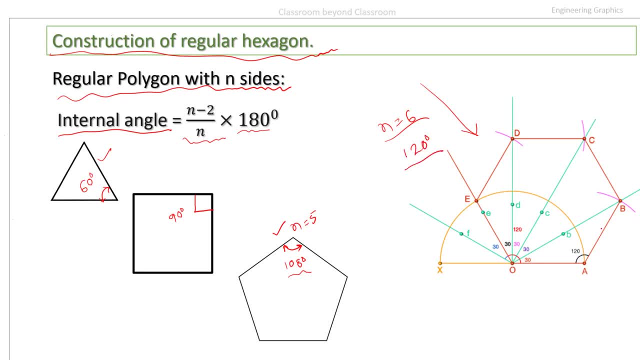 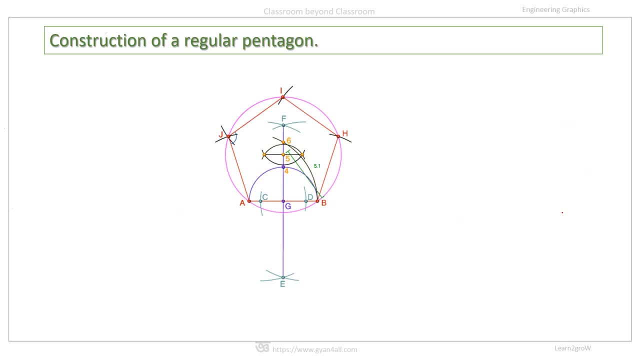 angle equal to 120 degree. This is the angle: 120 degree. So we'll construct this type of hexagon and, moreover, we'll also construct a regular pentagon by using proper engineering drawing methods. So let us dive into the next section of the. 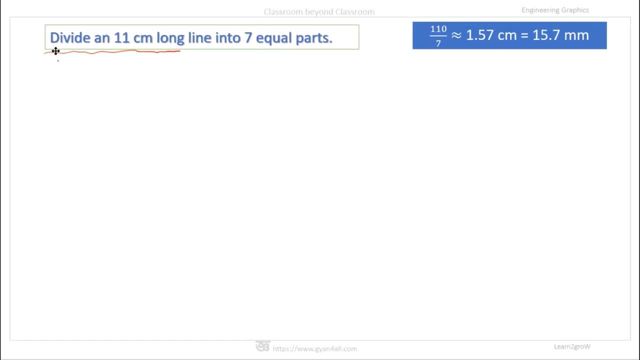 videos. So the line is 11 centimeter long and we have to divide it into 7 equal parts. Now if we divide 11 centimeter, or 110 milimeter, by seven, then we get the figure 1.57 centimeter, and that is. 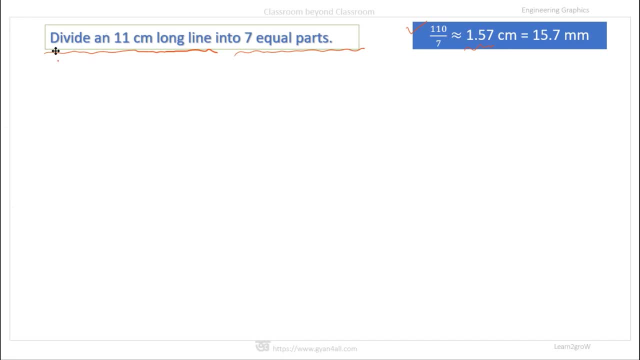 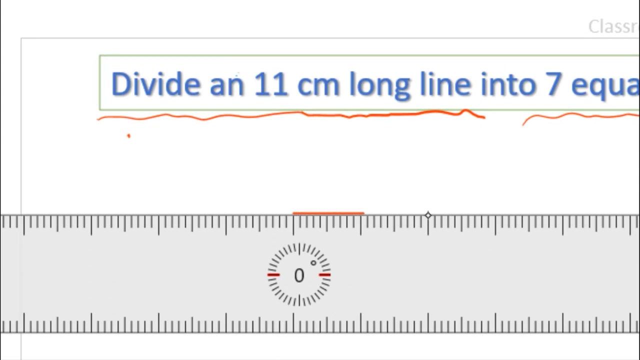 equal to 15.7 millimeter. By using a ruler it is very difficult to divide 15.7 millimeter. This is a centimeter millimeter ruler. So from the scale we can see the 15.7 millimeter is equal to something like: from here it is 10 millimeter and again 15. this is equal to 15 millimeter. then this is equal to 15.7 or so. 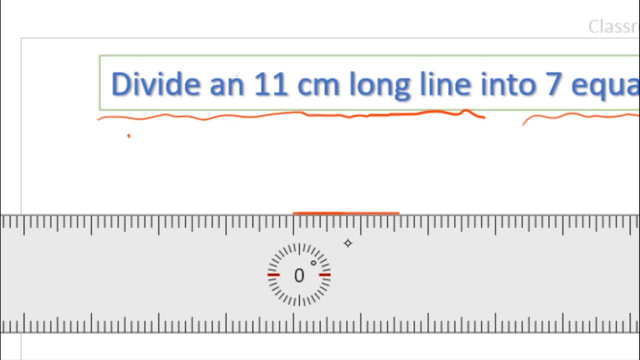 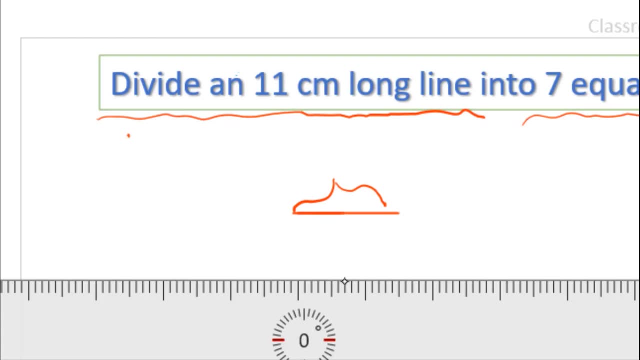 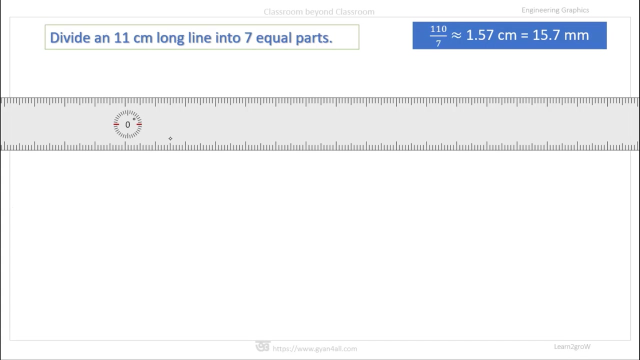 So it is not so easy to draw this type of line with accuracy, And for that there is a tactic to divide a line into equal parts by using scale, set, square and minute after. Let us first draw a line which is equal to 110 millimeter or 11 centimeter. 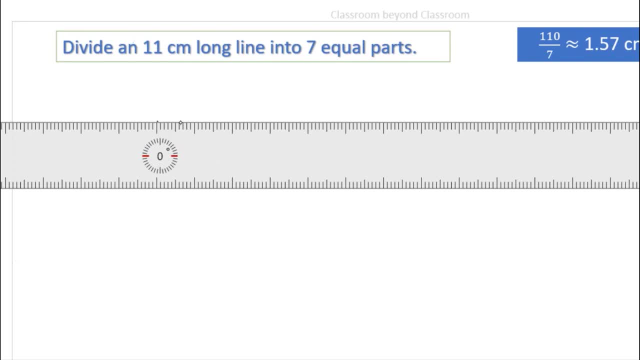 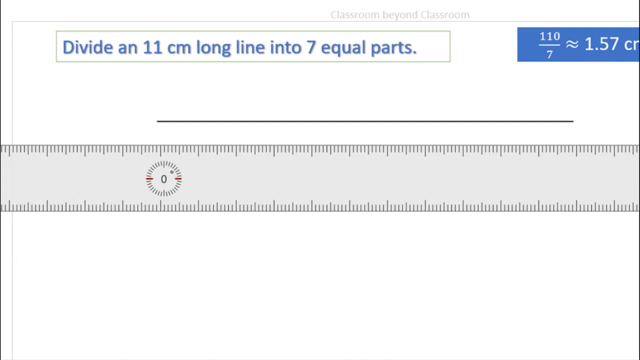 So we will start From here: 1,, 2,, 3,, 4,, 5,, 6,, 7,, 8,, 9,, 10, and this is 11 centimeter. So this is a line which is equal to 11 centimeter long. say then line is A, B. 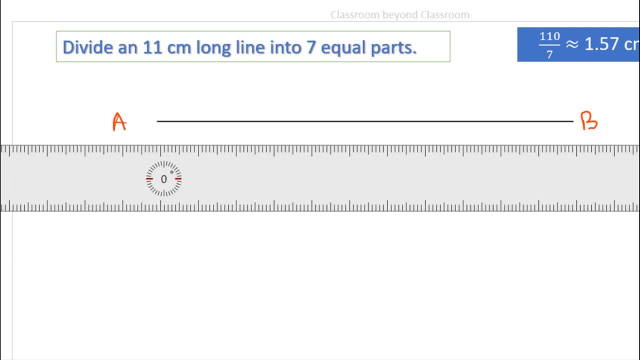 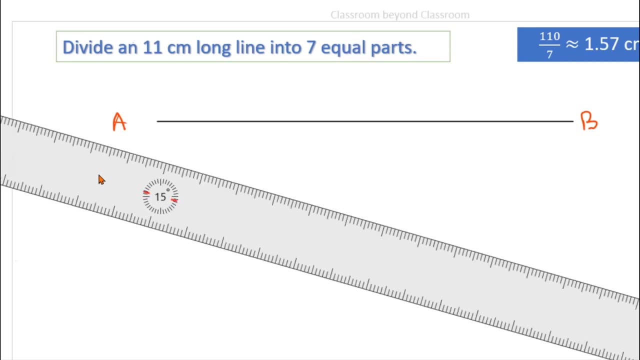 We are to. We are to divide the line A- B into seven equal parts. First, you have to draw the line A- B with the help of T square or mini drafter. Then, the next step, we are to draw an inclined line. 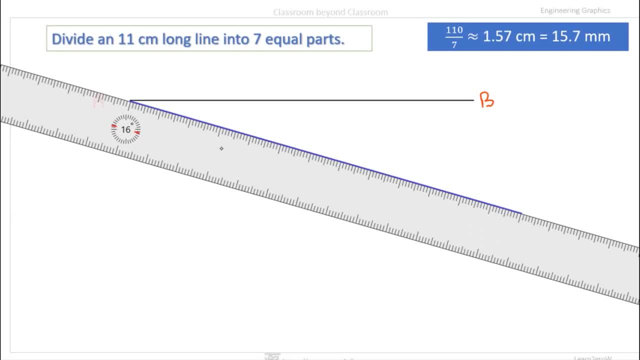 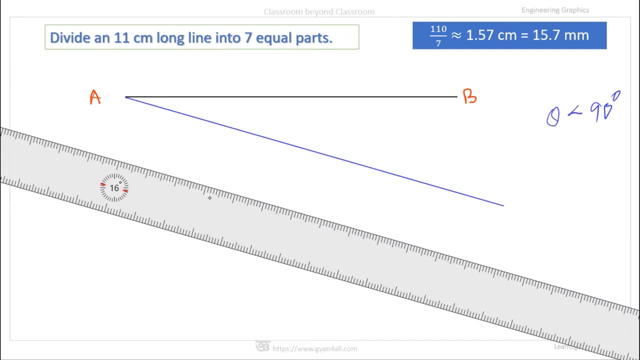 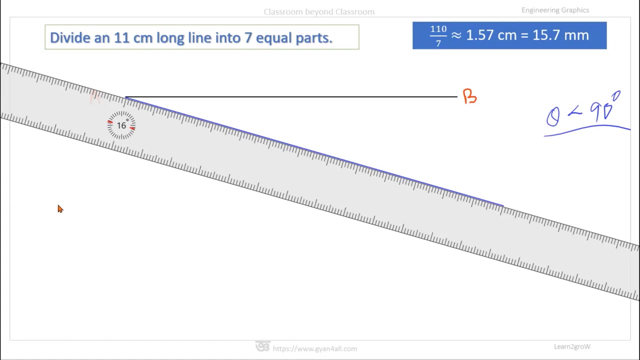 This is a line inclined to the line A, B, and this for this the angle of inclination should be. theta should be less than 90 degree. That means it is better if the angle is An acute angle. So by using a scale, we are to make seven equal divisions and while using a drawing sheet and set square, et cetera, you have to. you can use the divider and also use the ruler to divide seven equal divisions. safe in our case. I will divide it with the help of scale, scale only. 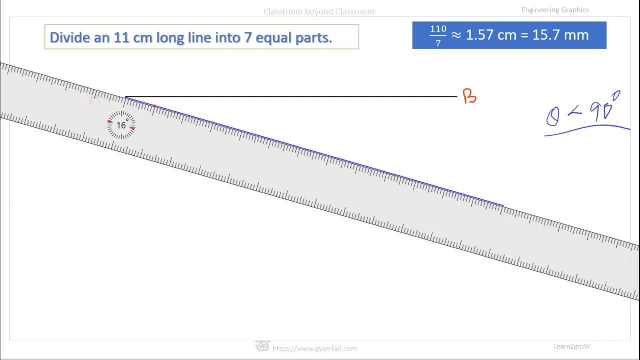 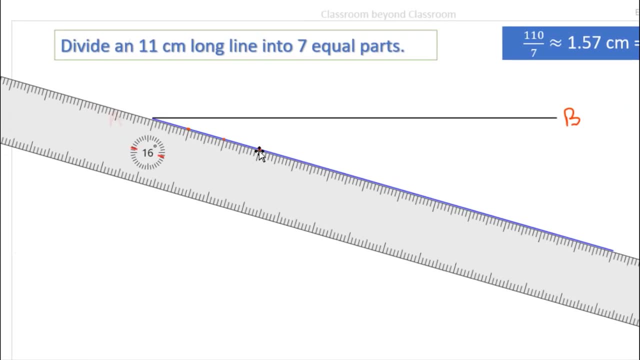 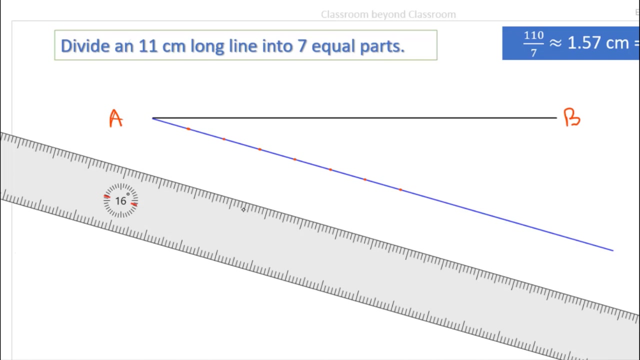 Suppose this is One, Two, Three, Four, Five, Six And this is seven. So these are all some equal divisions. Say: this is one dash, This is two dash, This is three dash, This is four dash, This is five dash. 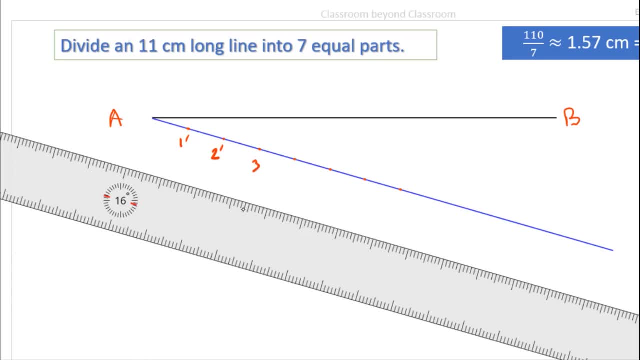 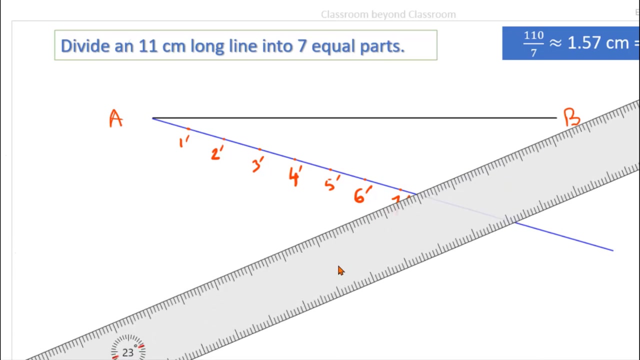 This is six dash. This is seven dash. Three dash, Four dash, Five dash, Six dash, Seven dash. We have seven equal divisions or parts. Now the next step is to join the seventh point with that of the point B. So remember, you have to use one mini drifter or a scale for this type. 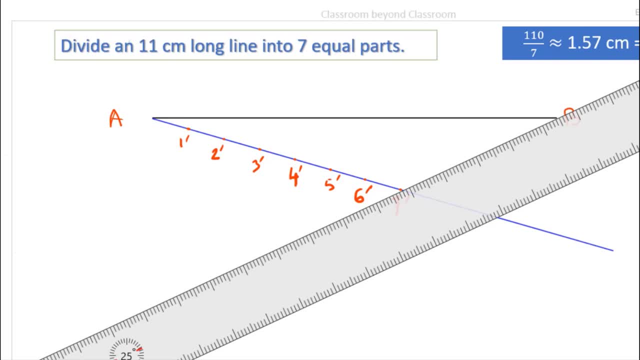 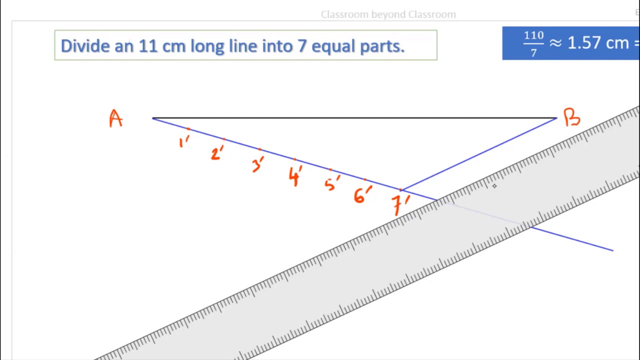 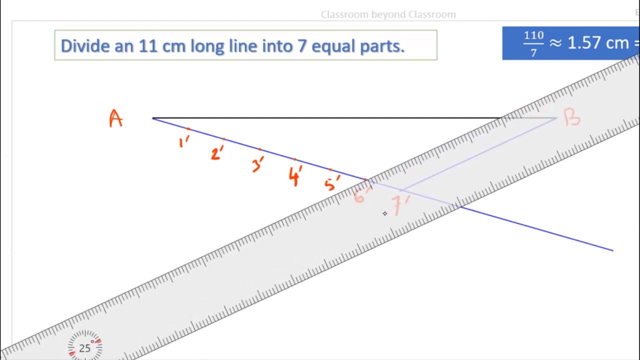 For a scale for this type of construction. First we will join this two point seven dash and B. Next, since we have got one line, now we can draw parallel lines parallel to the line seven dash B, And for that you can use mini drifter or set square, combination of the set squares, So this way you can draw. This is the second line. This is another parallel line. 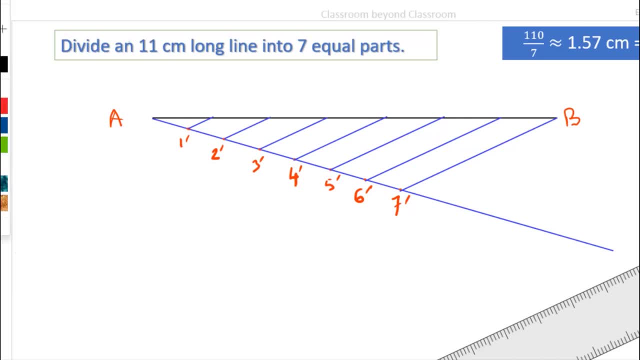 And therefore we get the equal divisions like 1,, 2,, 3,, 4,, 5,, 6 and 7.. So this way we can divide one line by drawing one incline line, A convenient length of line which can be divided easily with the help of a divider or with the help of a scale also. 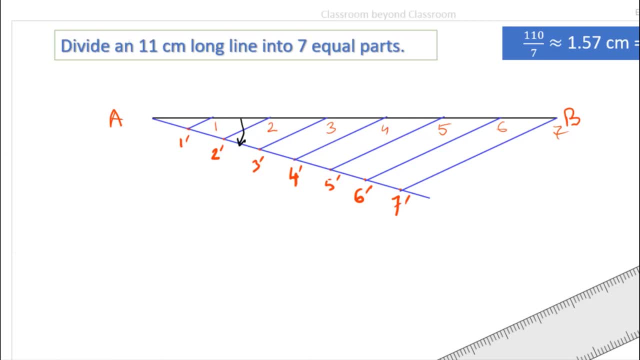 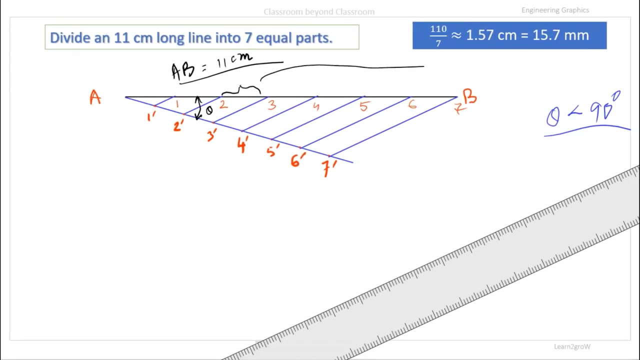 Remember- this is the second line. Remember- the angle of inclination should be less than 90 degree. That means it should be an acute angle. Better to have an acute angle less than 90 degree. You can draw 90 degree also. So this way we divide the line AB is equal to 11 centimeter And this each division is, approximately, is equal to 15.7 millimeter. 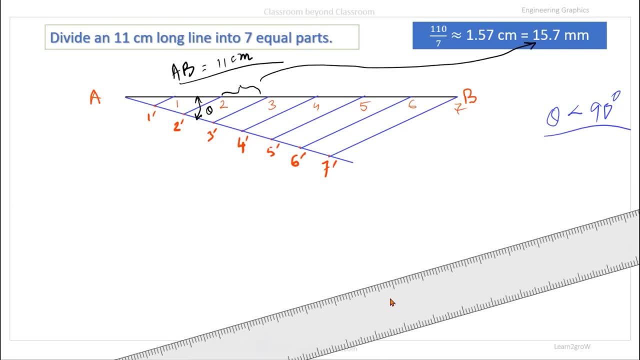 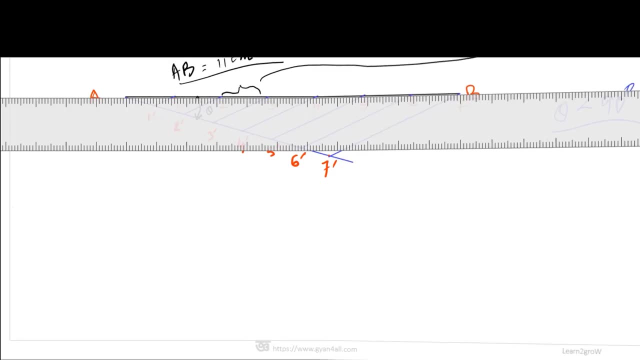 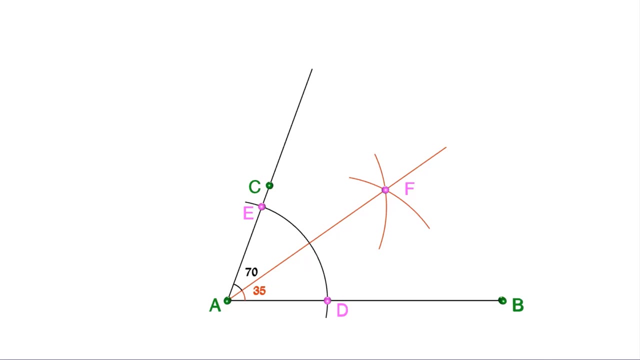 That we can check with the help of this ruler Also. you can see, this length is approximately is equal to 15.7.. Okay, Now we will try to construct an angle, say CAB, And that angle has to be bisected by a line, say AF. 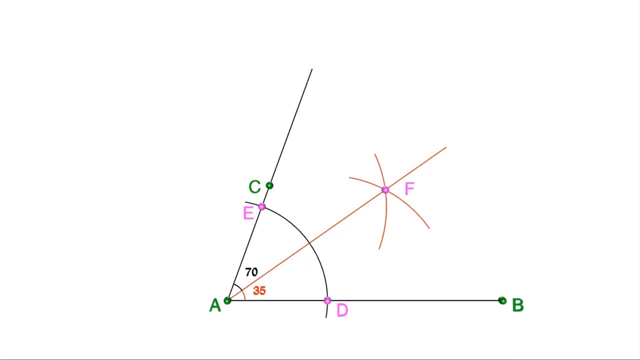 So the bisected angle FAB will be equal to 35 degree. So let us construct the angle CAB first. So let us construct the angle CAB first. To do that, we have to draw a line AB with the help of a scale T square or mini drafter. 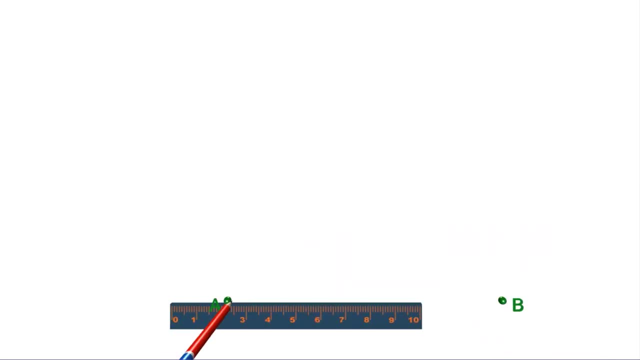 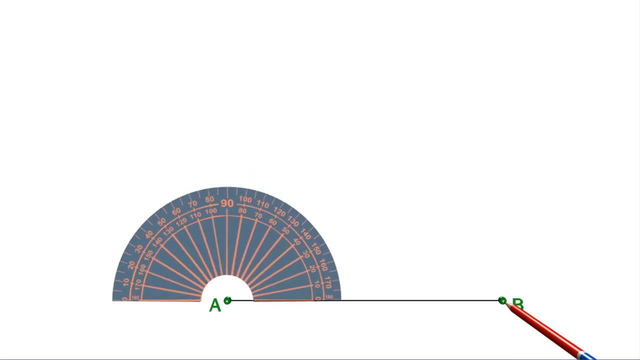 So locate the two points A and B and join AB with the help of mini drafter T, square or scale. Now measure an angle of 70 degree And locate the points C. Now join point A and C And this CAB is 70 degree now. 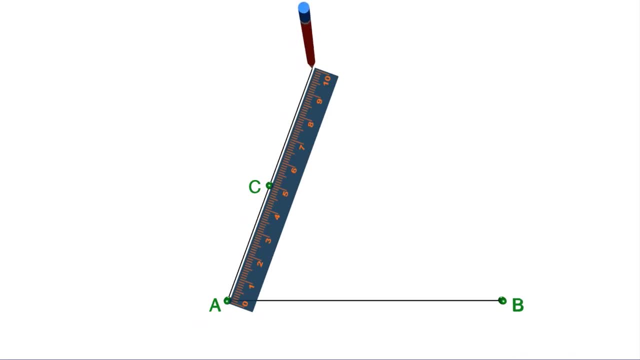 CA line can be extended beyond C also. Now, with the help of a protector, we can check whether the angle is 70 degree or not. This is 70 degree Now. taking A as a center, Draw an axis, It is 70 degrees more in front. 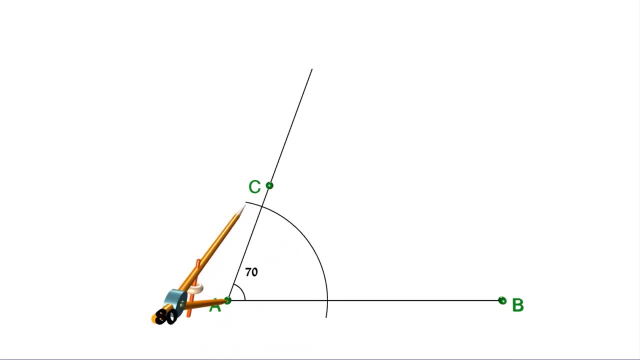 arc to cut the previous two lines at a point, D and E respectively. Remember this radius can be taken conveniently and, taking D as the center, draw another arc with any radius and with same radius as previous. draw another arc, taking E as center, to cut the previous arc. Suppose both the arcs cut at a point F. 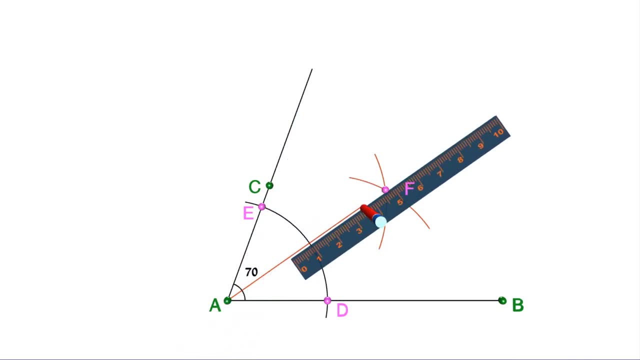 so join the point A and F and it can be extended beyond F So we can measure the angle FAB with the help of a protector, and this is 35 degree. that means the line fa bisect, the angle cab and the angle of bisection is 35 degree and original angle was 70 degree. this way we can. 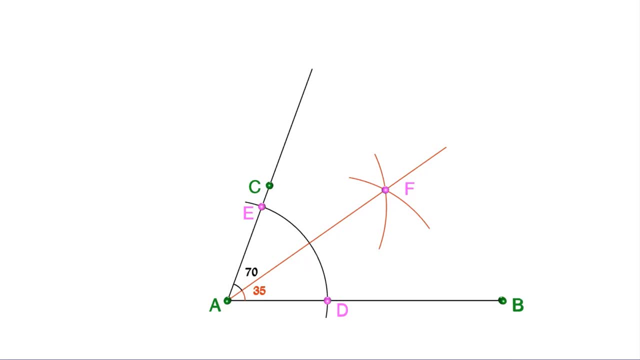 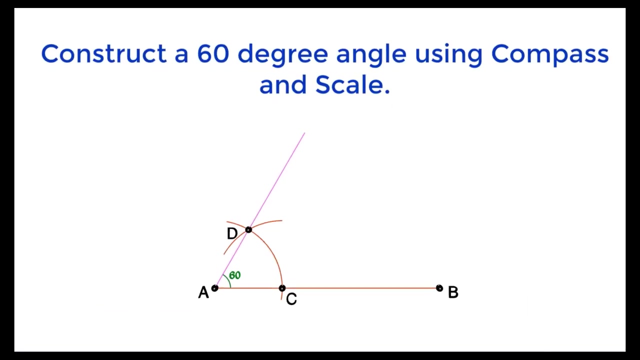 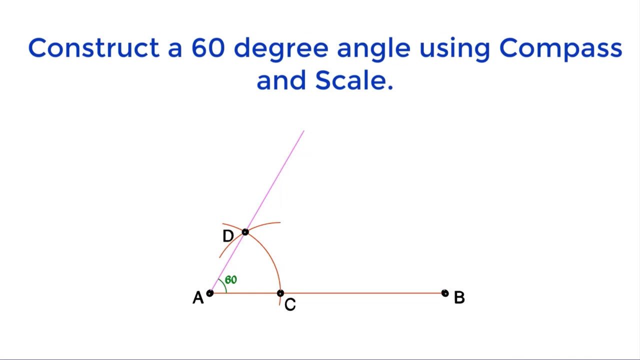 bisect any angle with the help of scale, t, square or mini drafter and compass only. now we will construct a 60 degree angle with the help of compass and scale only. we have to construct an angle d, a, b which is 60 degree and to use the compass and scale only. 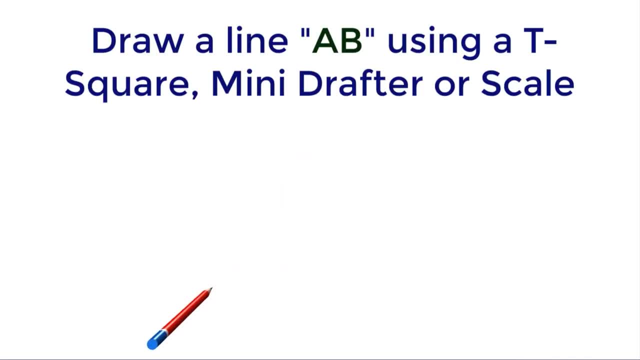 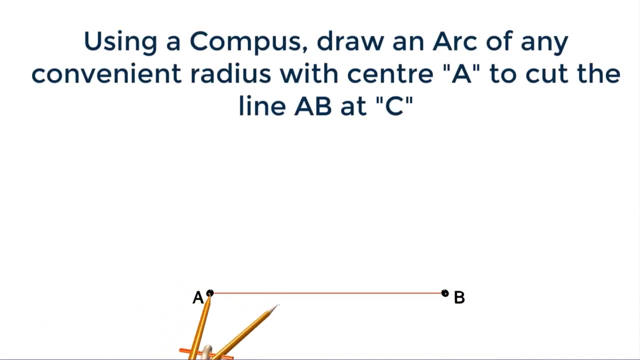 to do that, first we will draw the line a b. so locate the point a and b on the drawing set and, with the help of t square, mini drafter or scale, draw a line a b. line a b now, taking a as a center and taking any radius, draw an arc. 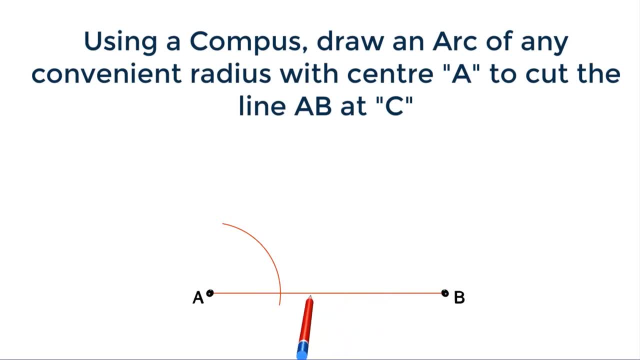 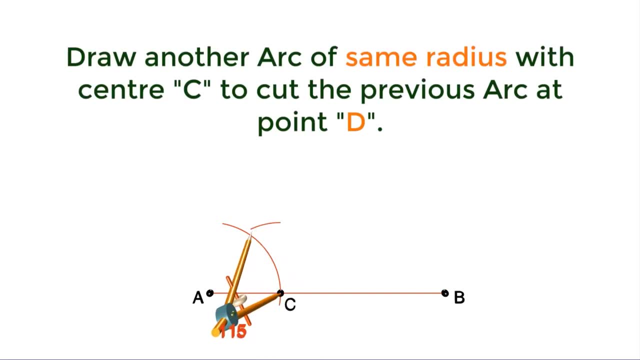 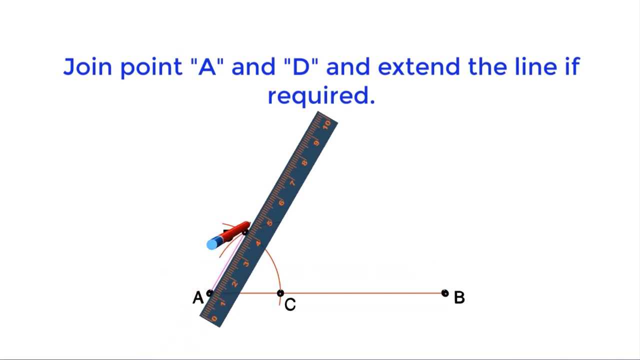 to cut the line a, b at a point, say c now, taking c as a radius and same radius as the previous. draw another arc to cut the previous arc at a point, say d now, join a, d and extend it. now, with the help of a protector, we can. 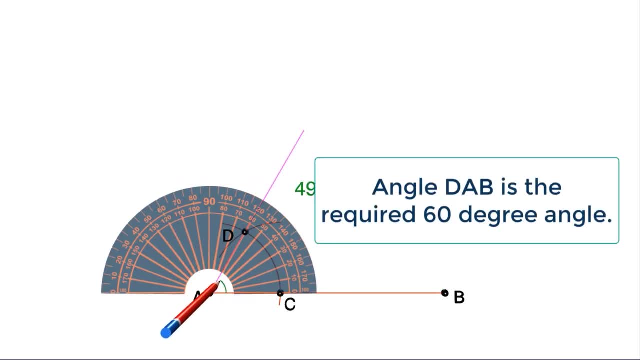 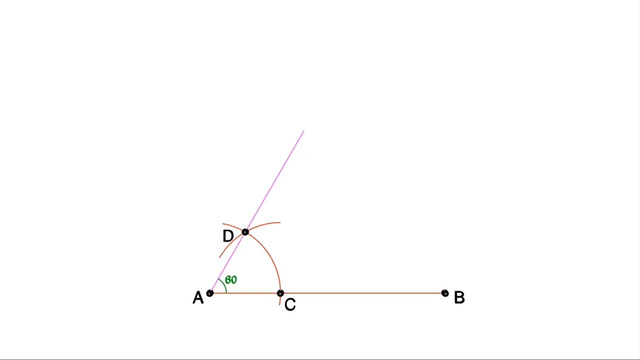 measure this angle, d a, b is equal to 60 degree, so this way, we can construct a 60 degree angle. with the help of compass, moreover, we can construct 30 degree angle, because by bisecting the 60 degree angle, we can construct a 30 degree. 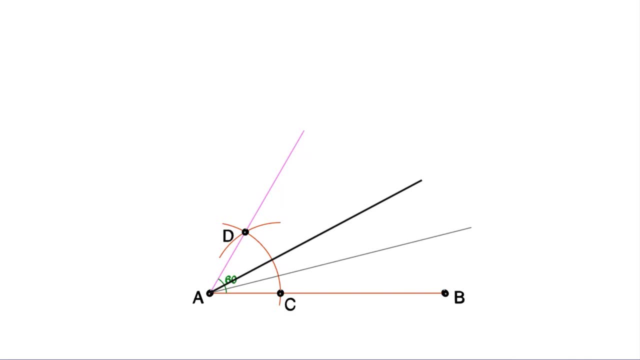 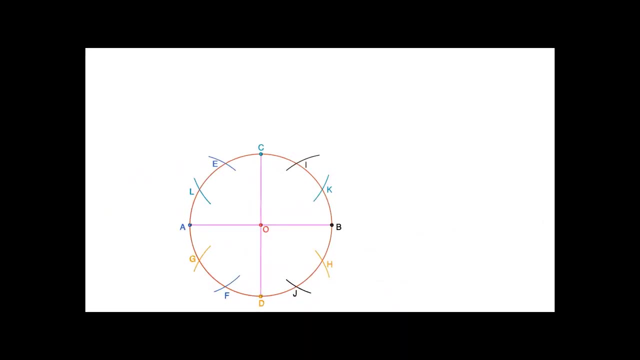 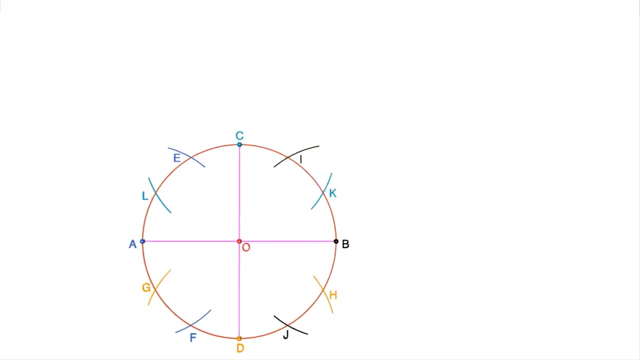 angle also. even we can construct 15 degree angle also by bisecting the 30 degree angle. okay, now we will draw a circle of six centimeter radius or 12 centimeter diameter. okay, we have a circle of 12 centimeter diameter or six centimeter radius and we have to divide. 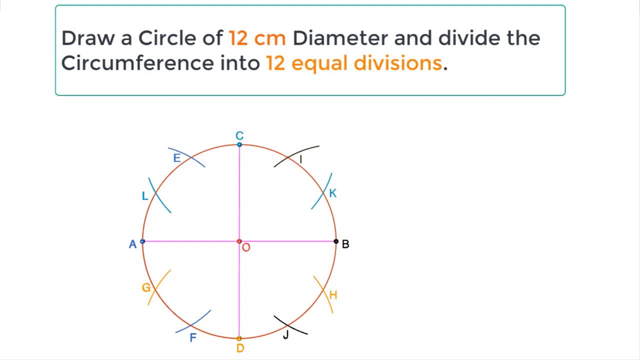 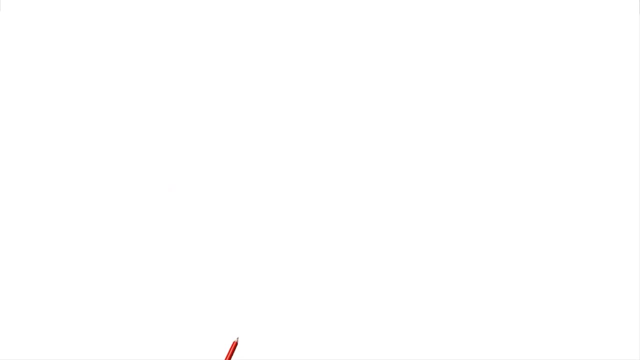 the circumference of the circle into 12 equal parts, and we'll do it once again with the help of a scale and compass. Now let us draw a circle first. Now, first, locate the center of the circle, O, and taking O as the center and 6 cm as radius. 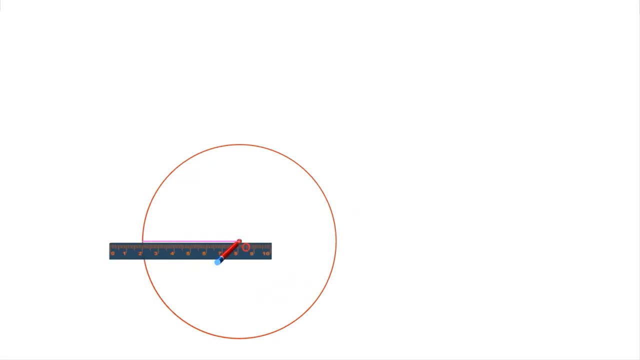 draw a circle whose diameter is 12 and draw the horizontal diameter like this with the help of a scale. Let the line be A and B. Both A and B are on the circumference of the circle. Also, draw another particle diameter of the circle and name it as C and D. 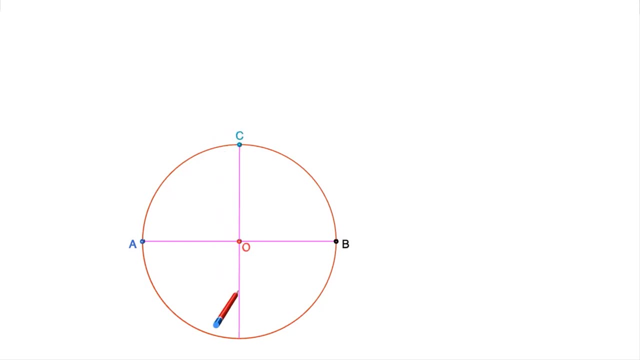 Now let us draw another circle. So we get 4 points till now. Now, taking A as the center and 6 cm as the radius, that means radius of the original circle- draw two arcs to cut the circle at point E and F. Again, taking D as the center, draw two more arcs. 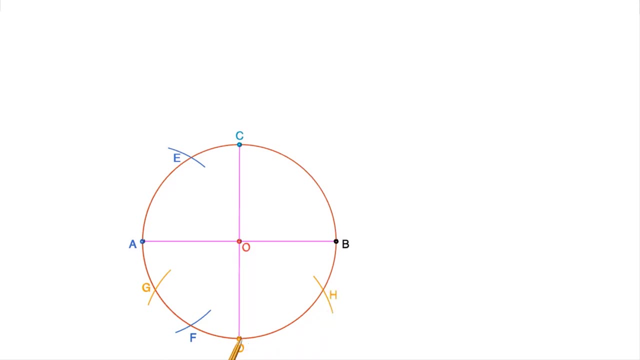 Cutting the original circle at point G and H. For all these arcs the radius should be 6 cm. that means radius of the original circle. So, taking B as the center, we get two points, I and J. Again, taking C as the center, draw two more arcs cutting the original circle at point 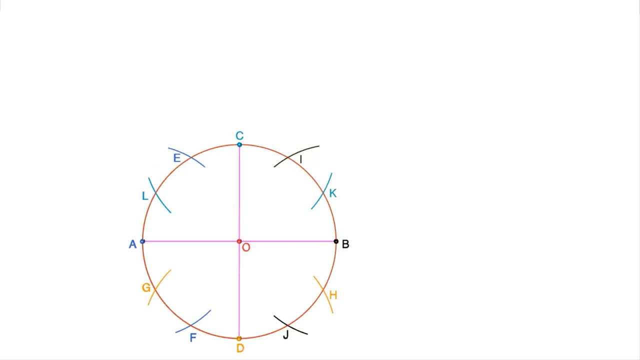 K and L, Again, taking L as the center, draw two more arcs. so we get 12 points: A, B, C, D, up to L. That means we have divided the circumference of the whole circle into equal parts, And this parts are like Lt, est, le. these are the segment of the whole circle. 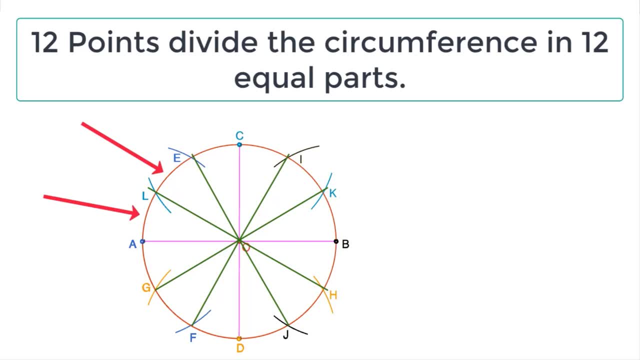 le is the arch, plec is another part of the circle that is arch. So this way we can divide the circle like this. That means, after so many times we have divided sauce balls into equal parts, like us, and acd circumference of a circle with the help of compass and scale into 12 equal parts. 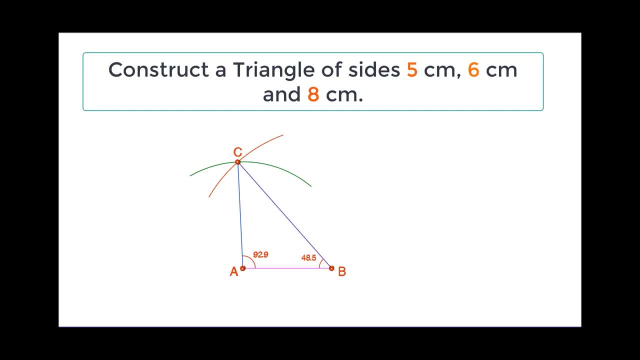 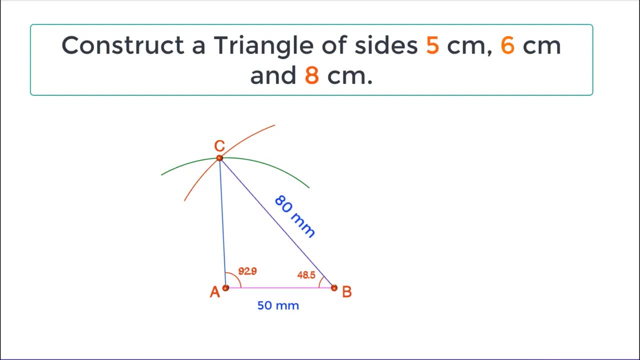 okay, now we are to construct a triangle ABC. the side AB should be 5 centimeter long and side BC is 8 centimeter long and side AC should be 6 centimeter long. that means the three sides of the triangle are given and we are to 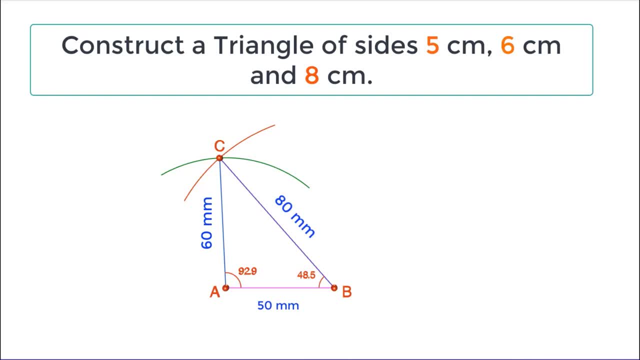 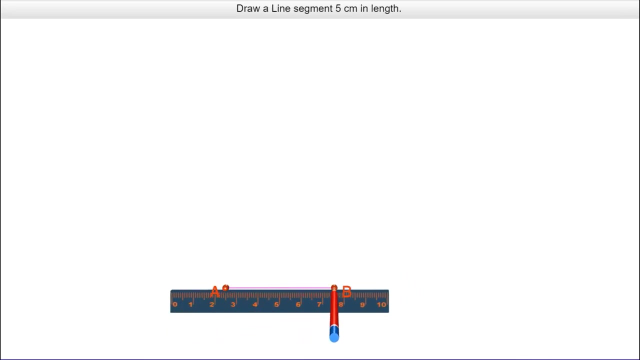 construct local triangle. so we start with line AB first. so construct a line AB which should be 5 centimeter long. so AB is five centimeter long line now, taking A is the center, draw an arc with six centimeters and a line AB should be 7 cm and tired. another line AB should be: 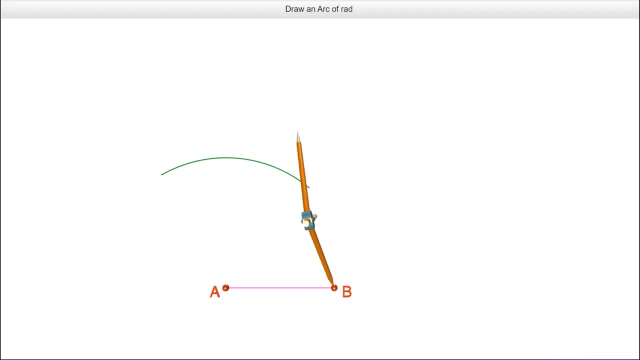 radius and, taking B as center, draw another arc whose radius is 8 centimeter long. now both the arcs cut at a point. say C, now join AC, which is equal to 6 centimeter, and join BC, which is equal to 8 centimeter. so this way we construct. 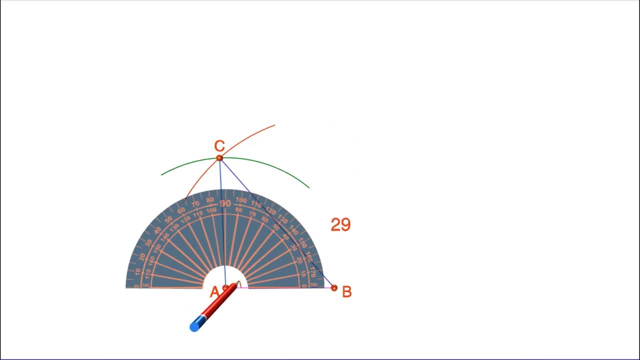 the triangle. we can also measure the angle if required. the angle is approximately 93 degree, that is actually 92.9 degree, and angle ABC is equal to 48.5 degree. so we have constructed the triangle with sides a vehicle, 25 centimeter, AC equal to 6 centimeter and DC is equal to 8. 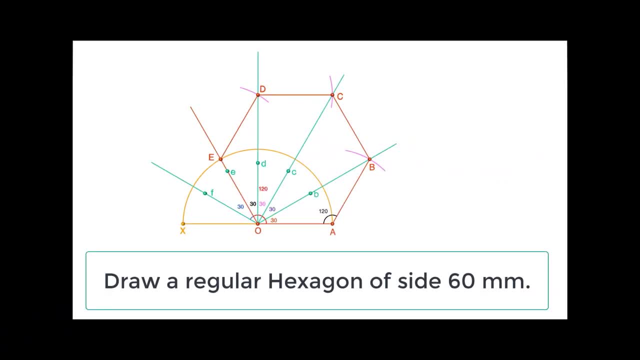 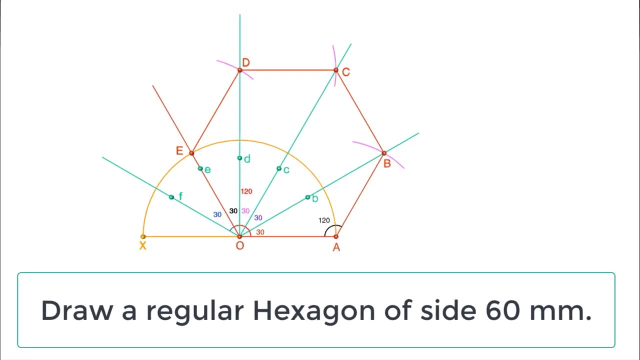 centimeter. okay, now let us draw one regular hexagon of side 6 centimeter, as you know, as semicircle has total 180 degree and the internal angle of a regular hexagon is 120 degree, and from that principle will draw the regular hexagon. first let us complete. 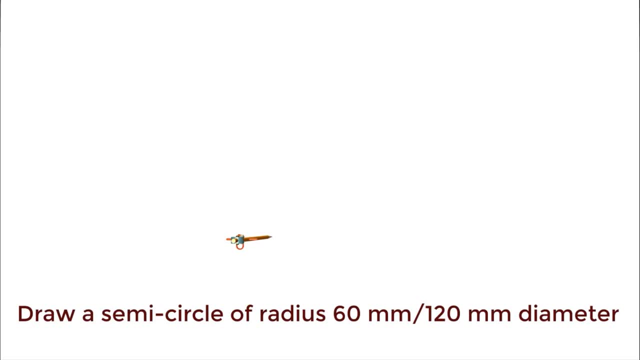 regular hexagon. first let us complete construction of a semicircle. Draw a semicircle and O is the center of the semicircle. We can complete the semicircle by joining the point A, O and X. So OX is radius of the semicircle, which is 6 centimeter, and we can extend. 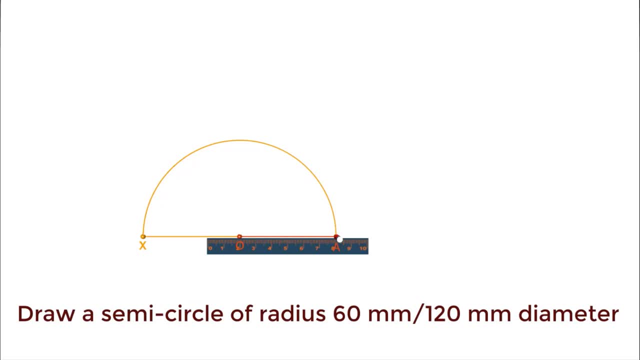 it from O to A, So AX or XA is 12 centimeter. Now we'll locate a point B at an angle of 30 degree with OA and extend this line. Similarly, we'll draw another 30-degree angle. First, locate the point C at an angle of. 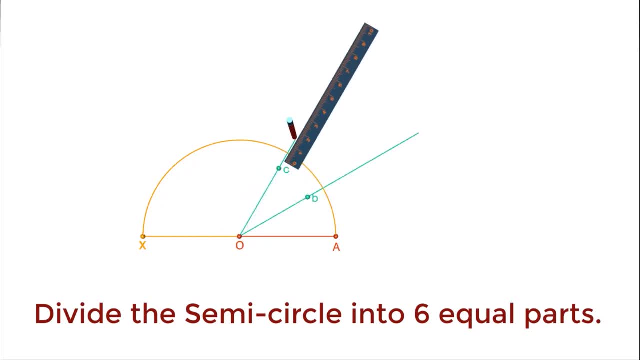 30 degree with licensedchart And complete the line and extend it. Draw another line at an angle of 30 degree after locating the point D. So till now we have completed 90 degree. Another line at an angle of 30 degree. Locate the point E and extend it. 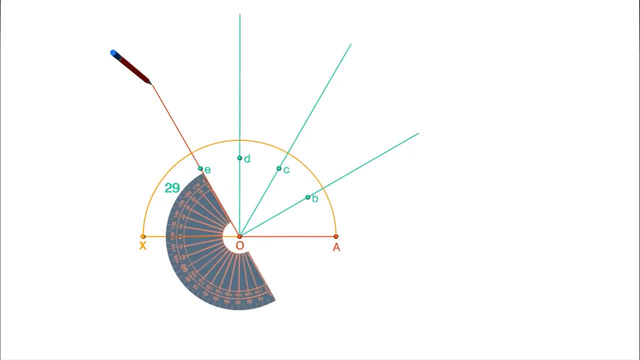 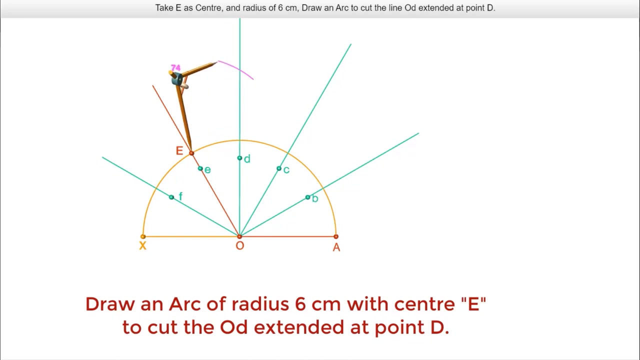 Another line at an angle of 30 degree. Locate the point F and extend the line. Now OE extended this line. Curse the semicircle at point E And, taking E as the radius, Draw one arc Taking 6 centimeter radius and this arc will curve the semicircle. 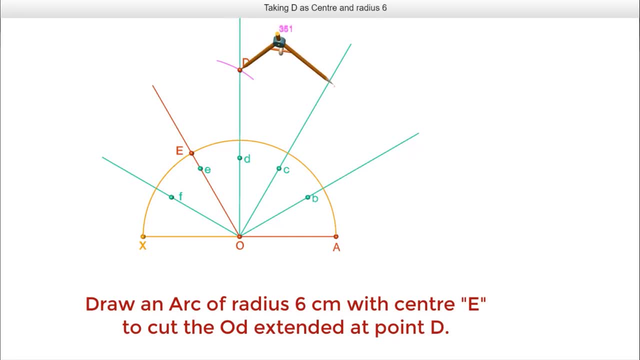 Cut the OD extended line at point D. Now again, taking D as the center and 6 centimeter radius, Draw one arc to cut the OC extended at point E. We can take C as the center or A as the center. In both the cases we will get a point B. 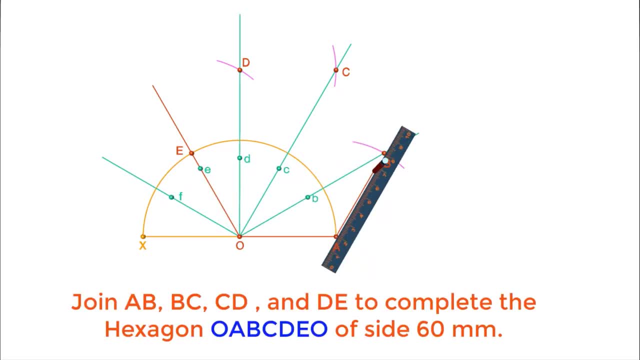 Now we join each point A, B. This is one of the sides of the regular hexagon. Join B, C, another side of the hexagon, Then C- D, another side, And D- E is the closing side of the hexagon And this completes the hexagon. OA, AB. 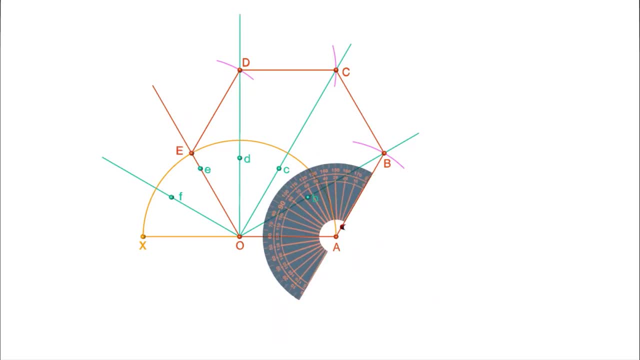 Also select both points: AU, RB and ED. You can suggest interesting angles to each point. Now we can measure the internal angle of a hexagon from 20 Ends. We can also measure the individual angles of each point, Which is 30 degree for each division. 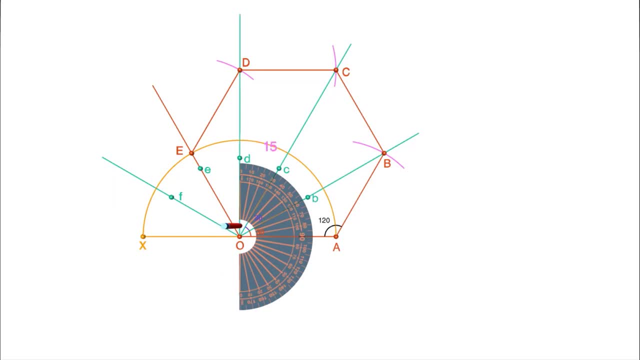 This is 30 degree And this is also 30 Degree and this is 30 degree. so this way we divide the semicircle. that means 180 degree, and from OA to OE this angle is also 120 degree. that is another internal angle. so this way, by 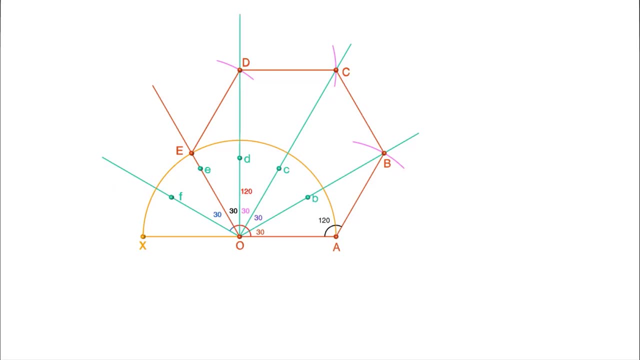 constructing a semicircle first and dividing the semicircle in six equal parts. if we want to draw the Pentagon, then we'll divide the semicircle into five equal parts. if we draw heptagon, then we'll divide the semicircle into seven equal parts and accordingly we'll complete. 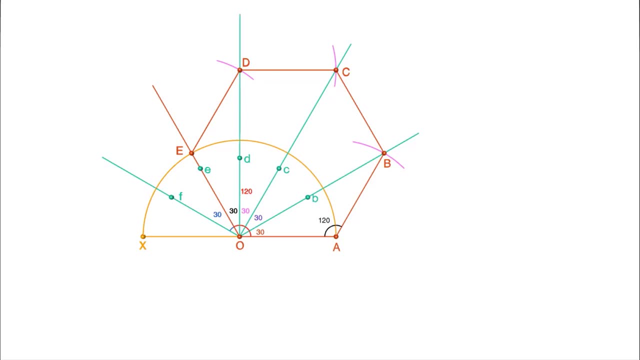 the polygon. so it depends on the number of sides of the polygon. in our example we have completed the construction for n, equal to six, number of sides of a regular polygon. so if six is the number, then that is hexagon. now we'll construct a Pentagon. that means a regular polygon. 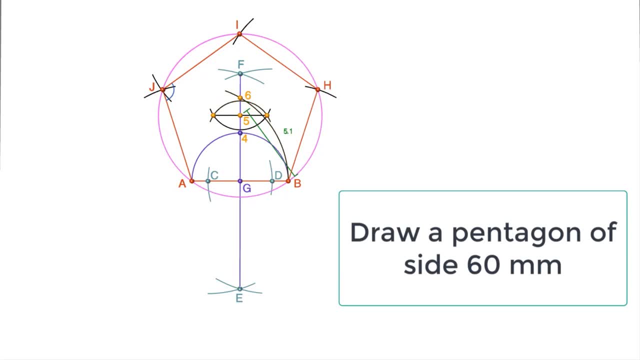 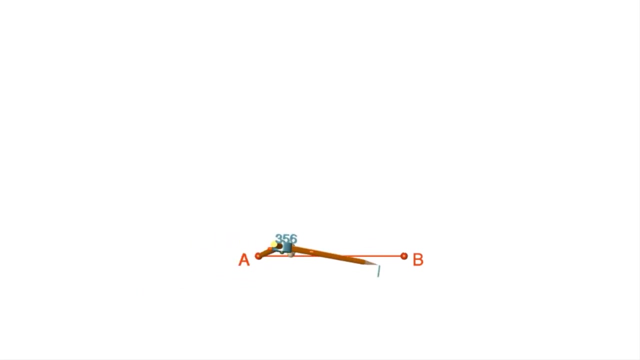 having five equal sides. we'll start with the line AB, that is, length of the line. AB is equal to 6 of the polygon, so let's draw a line. AB is equal to 6 centimeter. so let's look at the point A and B and we have to draw one perpendicular bisector of line AB. for that, by taking a radius less than equal, 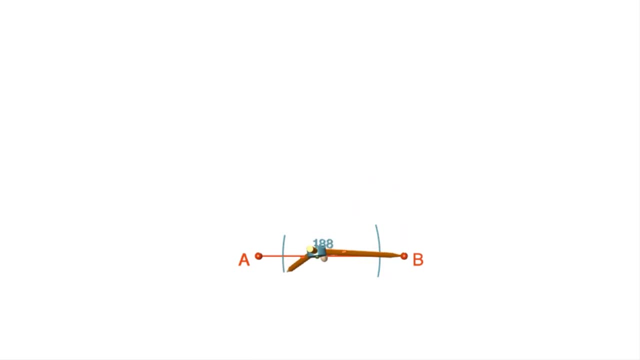 we draw two arcs to cut the line AB at point, say C and D. we'll construct a perpendicular bisector of line AB. now, taking C as the center and taking any convenient radius. draw two arcs on both sides of the line AB and taking D as a center. 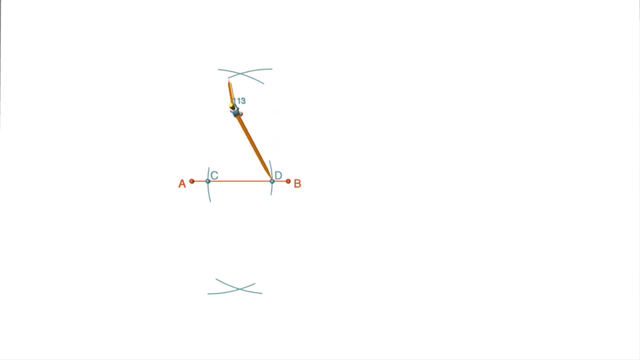 we'll draw two arcs to cut the previous arcs. let's the point of intersection of the two arcs be E at the bottom and F at the top. so let's join the point E and F and this line is the perpendicular bisector, so it bisects the line AB at. 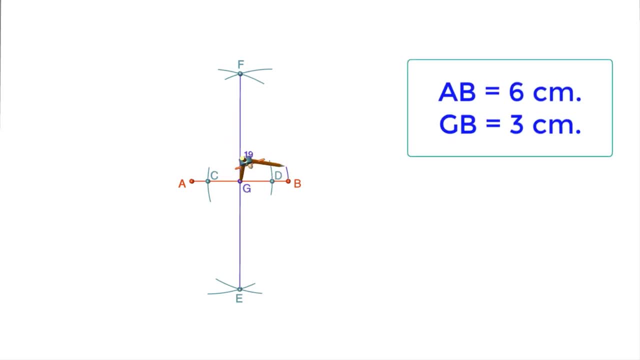 point Z. so, taking G in the center, let us construct a semicircle, and diameter of the semicircle is equal to AB. this semicircle cuts the perpendicular bisector at point four. Now, taking A as the center and AB as radius, let's construct an arc to cut the bisector. 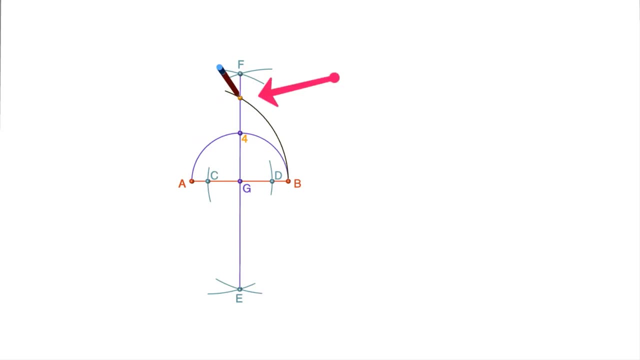 at point 6.. Now this segment of line 46 has to be bisected, and for that we'll use the compass. Taking 4 as center, let us draw one arc, Taking center as 4 and center as 6, both the arcs cut at two points and if we join these, 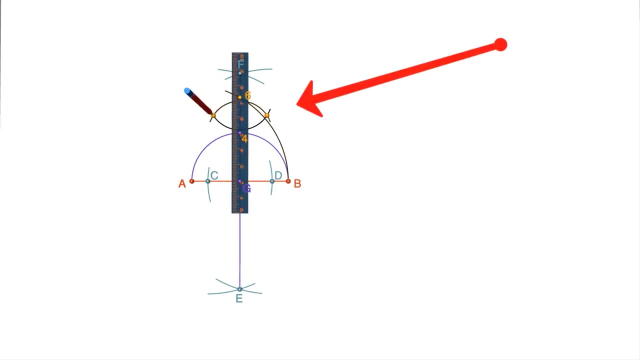 two points, then this line will bisect the section 46. The lines: This segment 46 is bisected by this line and this bisector cuts the line 46 at point 5.. So 45 is equal to 56. And from 5 to B, this distance is equal to 5.1 centimeter. 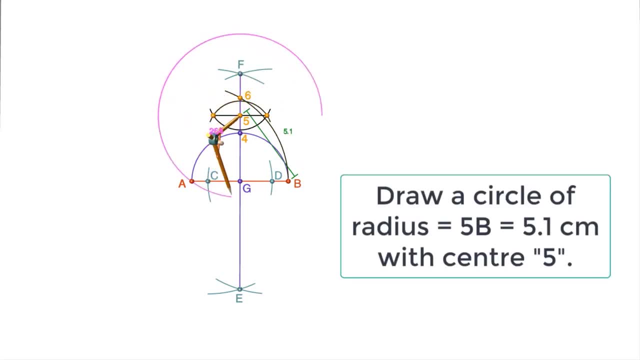 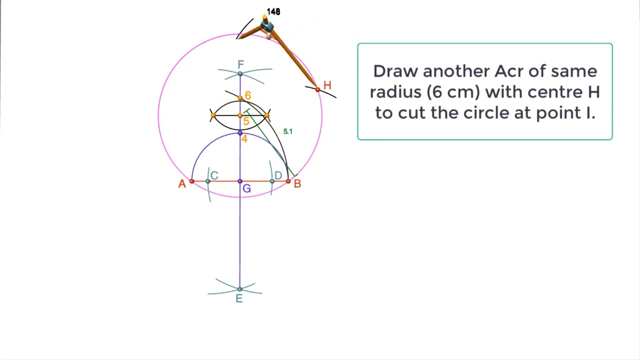 So, taking 5.1 centimeter as the radius, let us draw a circle, taking 5 as the center for pentagon. Now taking B as the center, let us draw an arc to cut the circle at a point and the radius should be is equal to 6 centimeter. that is the side of the pentagon. 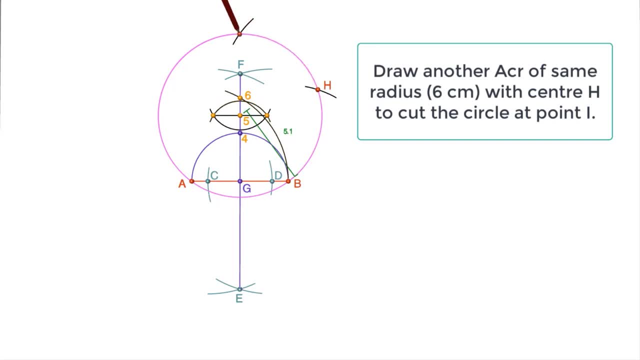 Similarly, taking H as the center, we'll get another intersection point I, and now also we can draw another arc from point A, That is the side of the pentagon. Similarly, taking H as the center, we'll get another intersection point I, and now also we can draw another arc from point A. 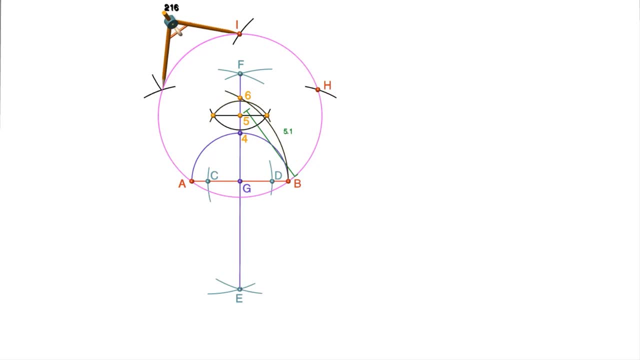 That is the side of the pentagon. Then also we can do the same thing taking I as the center. Both the arcs will cut the circle at a point. Let that point be Z. So now let us join the points B, H, which is one of the sides of the pentagon. 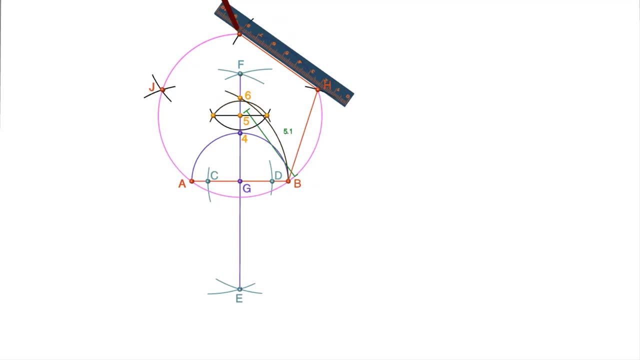 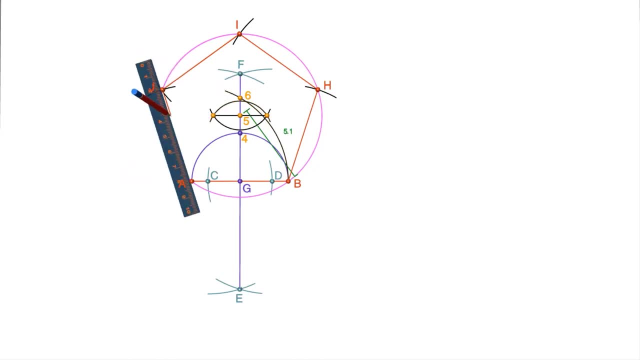 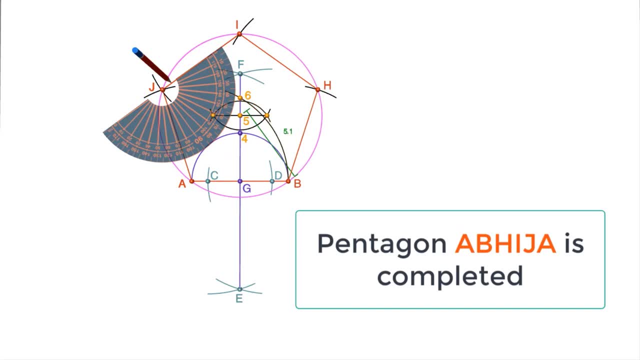 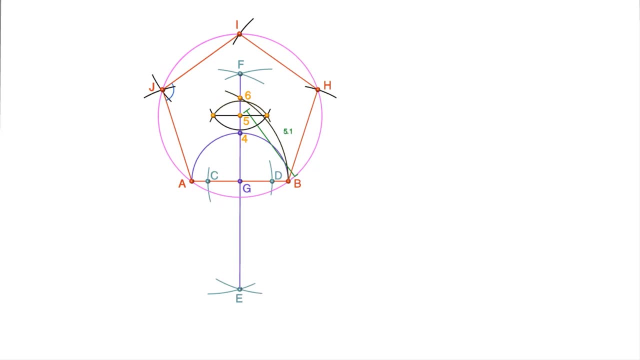 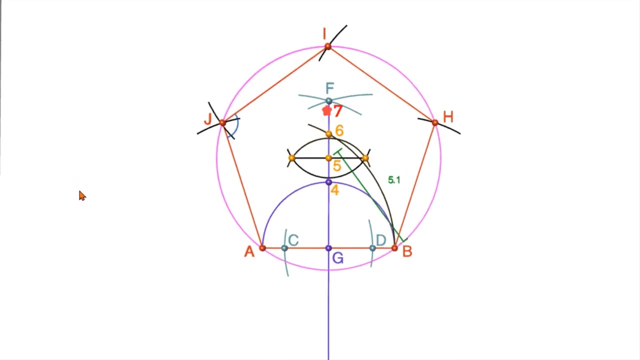